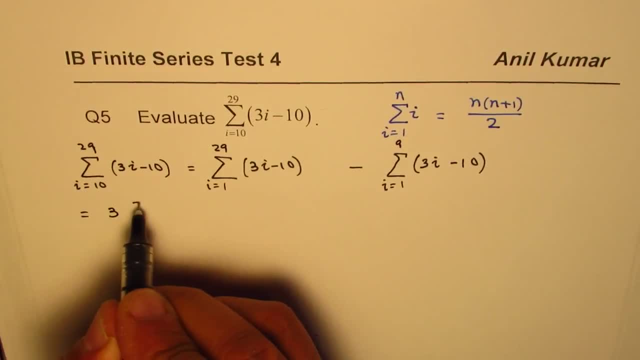 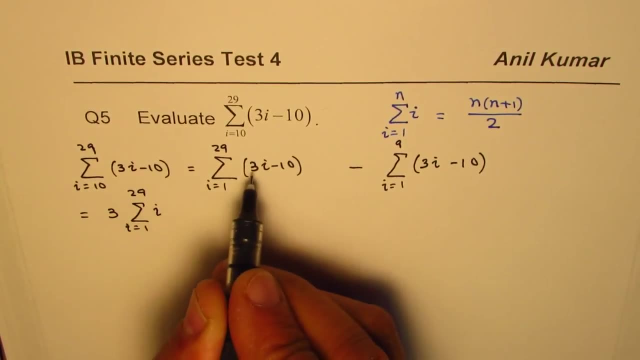 Let's open this up first. So it could be written as three times some from i equals to 1 to 29 of i. So I've taken out 3 minus now we'll do. there are 29. terms of 10 is a constant right, 10 times 1. you could write 10 here or outside with. 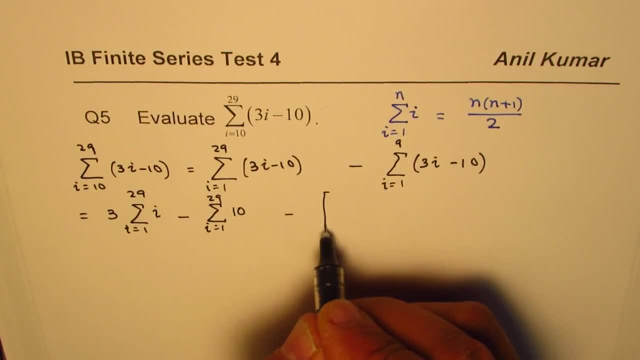 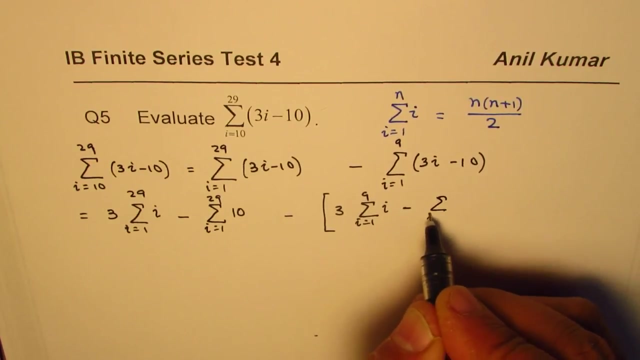 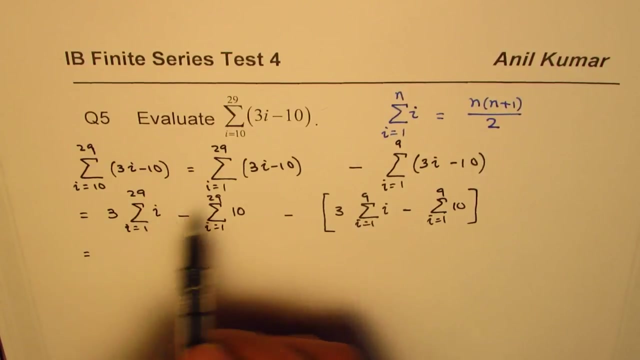 1 inside, minus this whole thing. so let me put this in brackets: it is 3: i equals to 1 to 9, for i minus 10 from, i equals to 1 to 9 of 10, right, so these are 10 numbers. so this sum, applying the formula i, is 29 for us. so that gives us 3 times 29. 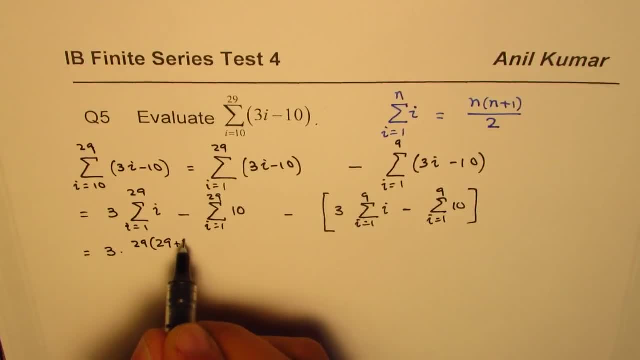 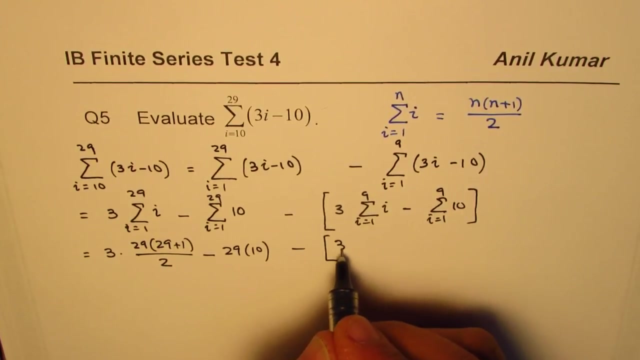 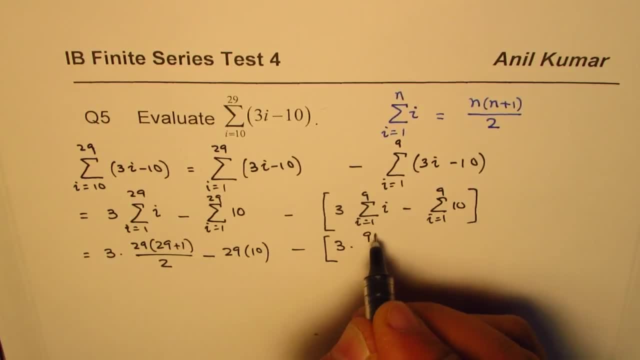 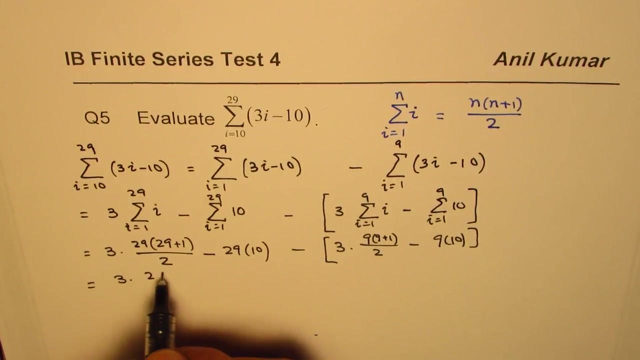 9 and it's 9 here, so it'll be 9 times. let me write 9 plus 1 divided by 2, minus their 9 tens, right, 9 tens. so that gives us 3 times 29 times 30 divided by 2. 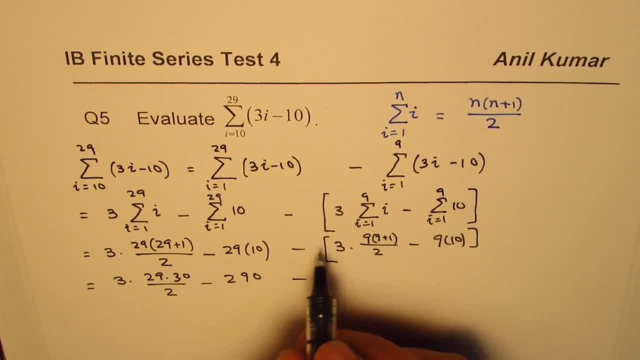 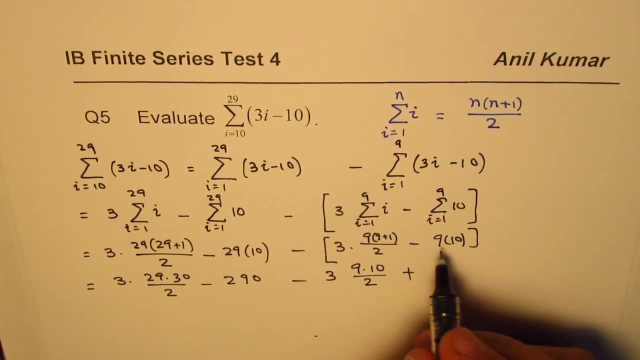 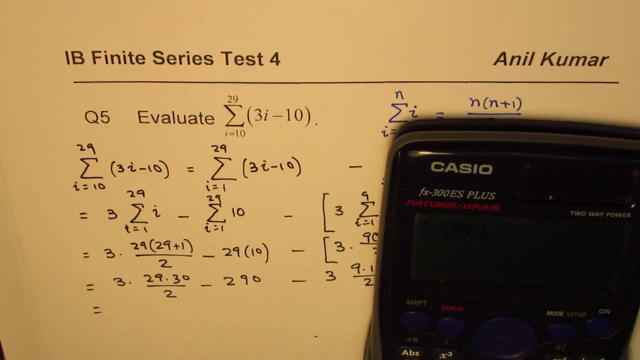 minus 290 minus. let's write down: 3 times 9 times 10, divided by 2 minus minus, becomes plus plus 90, right? so that is what it is. now we can actually use the calculator find the answer, right. so it is 3 times 29 times 30, divided by 2. 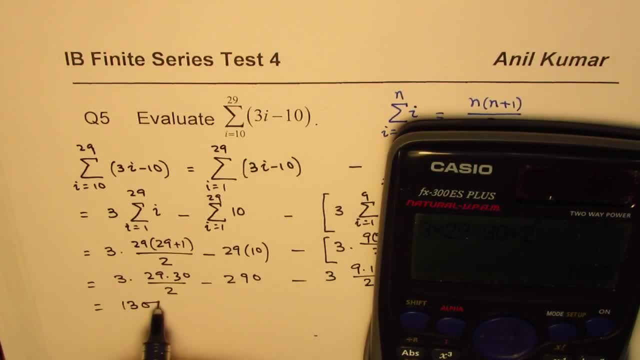 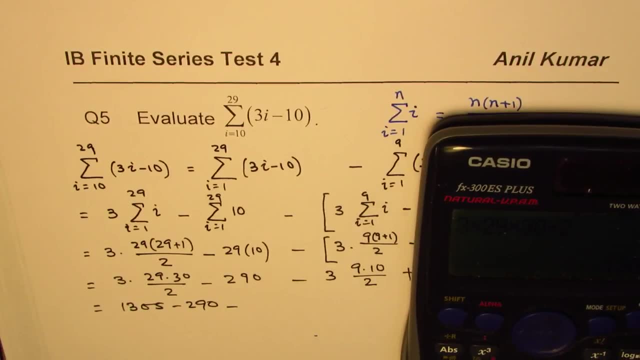 equals 2 plus 2. if you want, you can write the numbers also: 1305. okay, let's simplify this. and then do it: minus, 290, minus. we'll write 3 times 9 times 10 divided by 2 equals to 135 plus 90. right, so we have plus 90 here, and now let's.